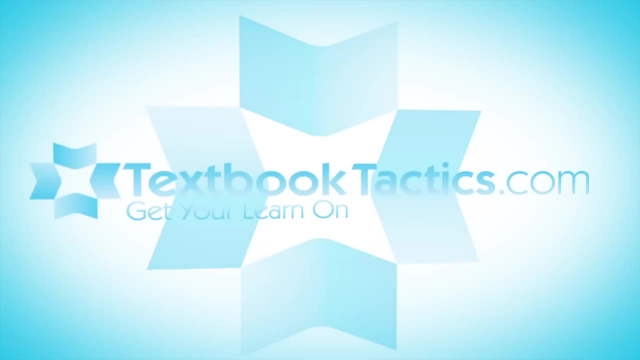 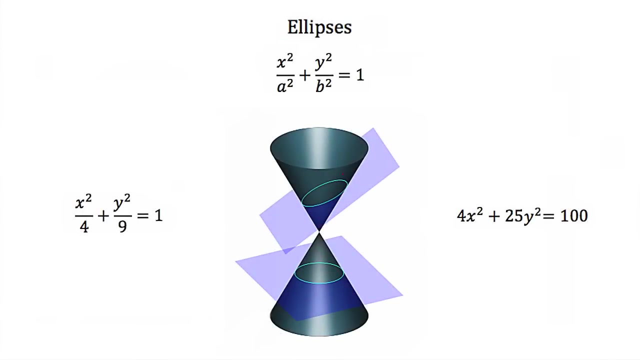 This is a tutorial on ellipses as conic sections. When we create a conic section that's shaped like an ellipse, we get it for when our intersecting plane cuts through our double cone in such an angle that when we look down at our plane, we have this stretched circle at the intersection of these two shapes. This stretched circle is an ellipse. Now the equation of this shape, if this shape has its center at the origin, can be written in a standard form and that standard form is x squared over a squared plus y squared over b squared is equal to one. An example of an equation of an ellipse written in standard form would be x squared over four plus y squared over nine is equal to one. An example of an equation of an ellipse that's not written in standard form would be four x squared plus twenty five y squared is equal to one hundred. Now we can tell that this is an ellipse because, like a circle, both my x squared and y squared terms are added together. We can tell that this is not a circle though because the coefficients on these two terms are different. 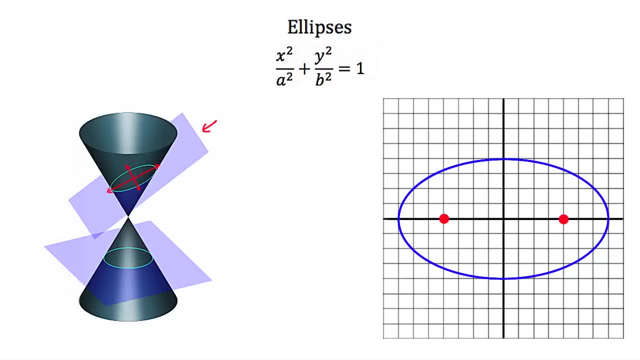 So if I take my double cone and I divide it by two, I get four x squared over b squared plus y squared over b squared. So I have a double cone and I intersect it with a plane at an angle so when I look down I see an ellipse. And if I were to imagine a coordinate axis on that ellipse, then I could take my coordinate axis and I could take my ellipse and I could put it on a graph and it would look something like this. Now like the focus of a parabola, an ellipse has two focuses or what we would say foci. And an ellipse is a special shape because every point on this ellipse has the same total distance to both of our foci. So for an example, if I chose this point on our ellipse and I measured the distance between that point and one of our foci and I called that distance d1 and then I measured from that point to our other focus and I called that distance d2. 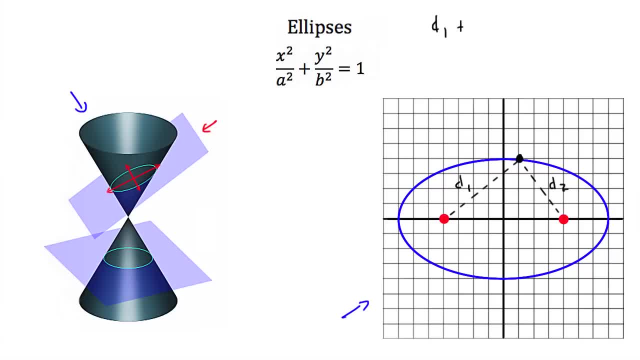 Then d1 plus d2 would be the same for every point on this ellipse. So if I chose a different point on the ellipse, say I chose this point and I measured to one of my foci and I said that distance was d3 and then I measured to my other focus and I said that was d4, well then d1 plus d2 would be equal to d3 plus d4. 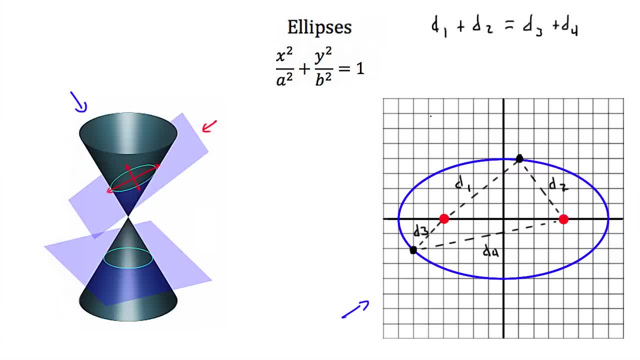 plus D4. In short, every point that makes this ellipse has the same total distance to both of these foci. So now let's talk about some terminology of ellipses. 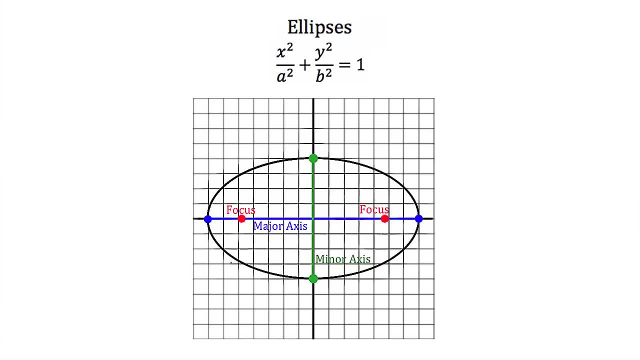 Every ellipse has two axes of symmetry. In this example ellipse, one axis of symmetry is the x-axis. Our other axis of symmetry that's the y-axis. Whichever direction our ellipse is stretched more that is our major axis. So in this example our major axis is the x-axis and our minor axis or the smaller axis is our y-axis. 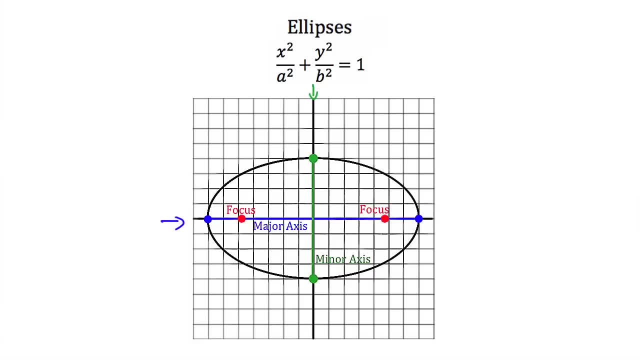 At the ends of both of these axes we have vertices. At the end of our major axis these are called major axis vertices or sometimes just vertices. 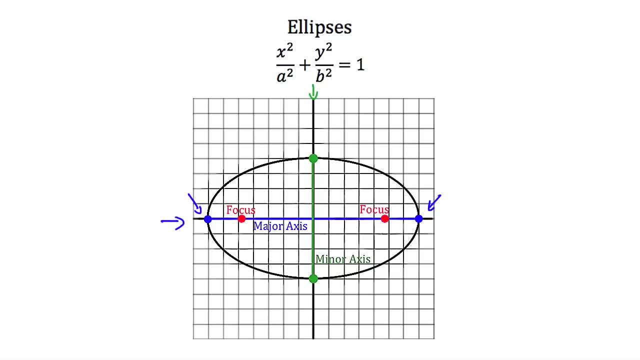 At the end of our minor axis we have minor axis vertices or sometimes these are called co-vertices. 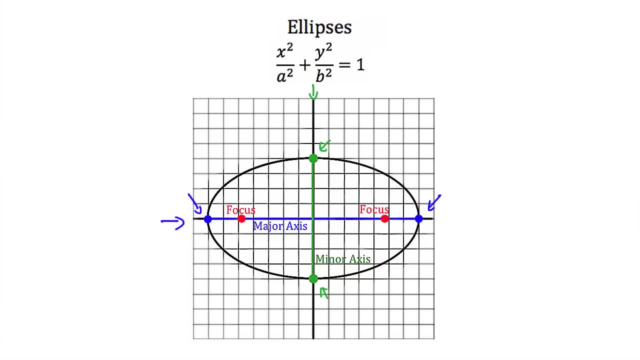 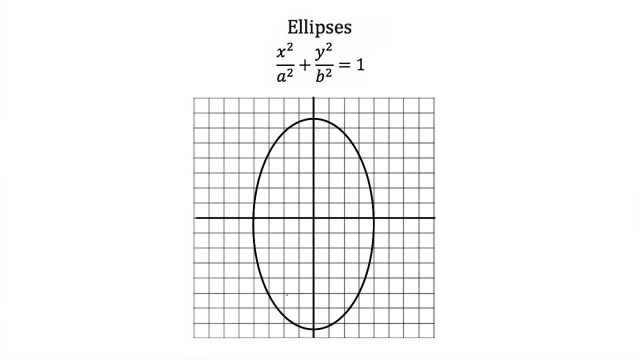 We also know about our foci. Our foci are always on the major axes. Now if our ellipse was stretched in the y-direction further than it was stretched in the x-direction, then the y-axis would be on the x-axis. 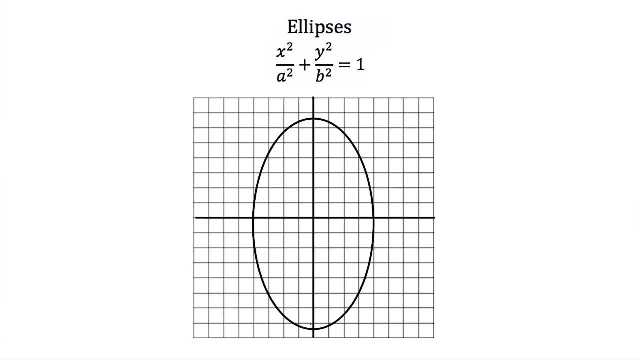 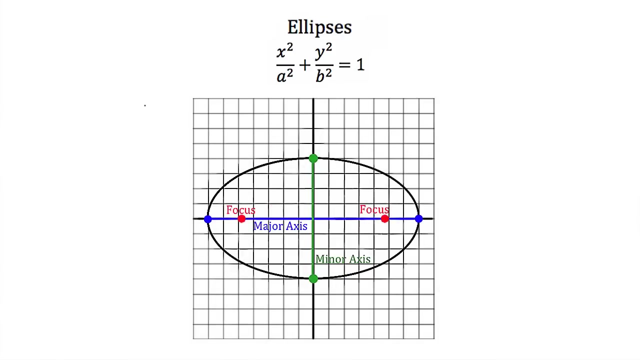 The y-axis would become our major axis and then the x-axis would become our minor axis. At the ends of our minor axes we would have our minor axis vertices or our co-vertices. At the end of our major axes these would be our vertices or our major axis vertices. Our foci are always on the major axis so now our foci would be approximately here. Now let's compare the shape of this graph to the standard form of our ellipse equation. Remember before I said a and b 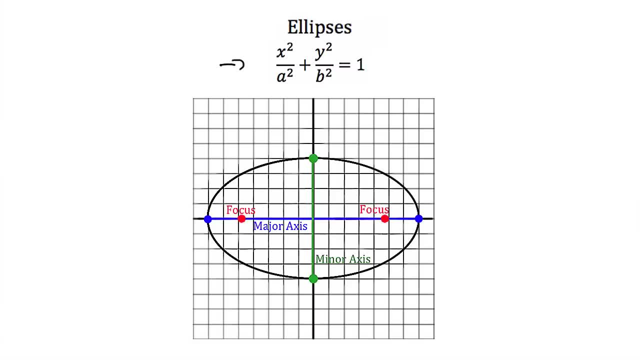 were constants that determine the shape of our ellipse. Notice that the a or the a-squared is underneath the x-squared term. That means that a is 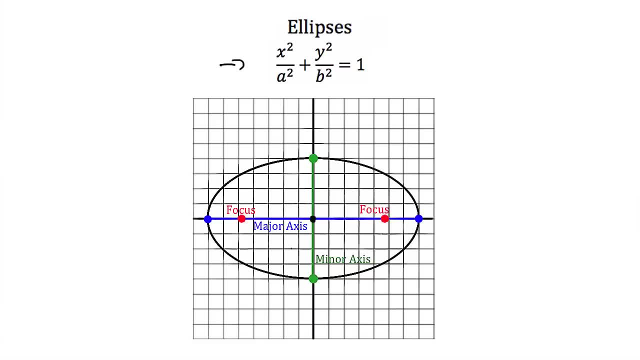 the distance from the center of our ellipse to the vertices in the X direction. This distance is A and this distance is also A. Notice that the B 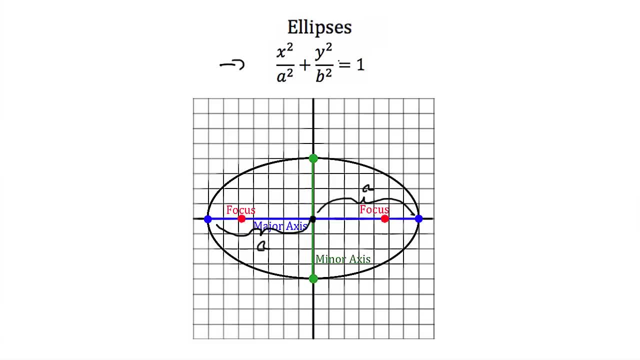 squared term is underneath the Y squared term. So the B distance is the distance from the center to the vertices in the Y direction. So this distance is B and 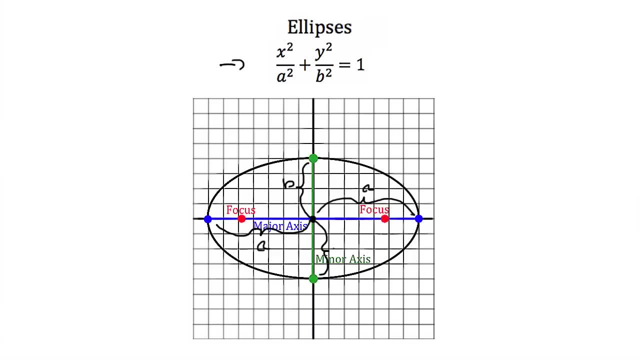 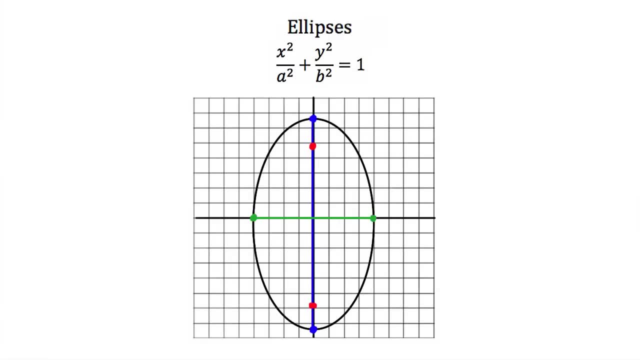 this distance is B. Now if our ellipse is stretched in the other direction, well then our A squared term is still underneath the X so this distance is still A and this distance is still A. 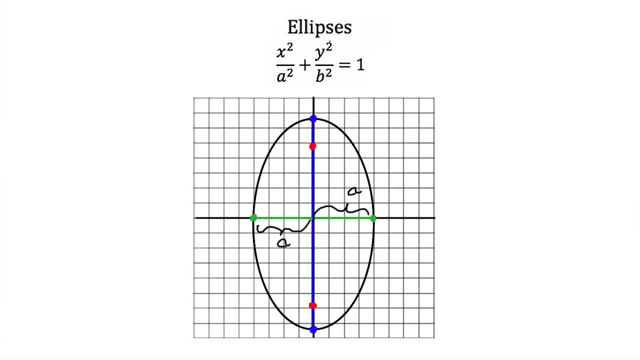 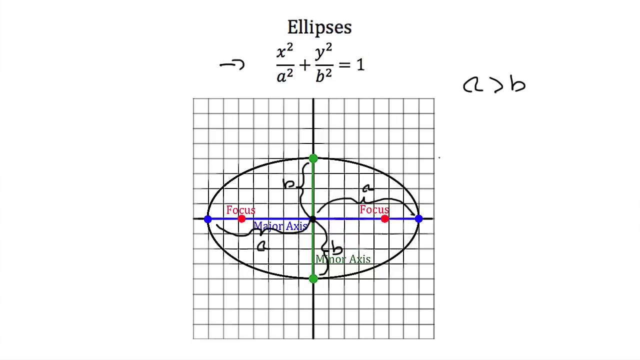 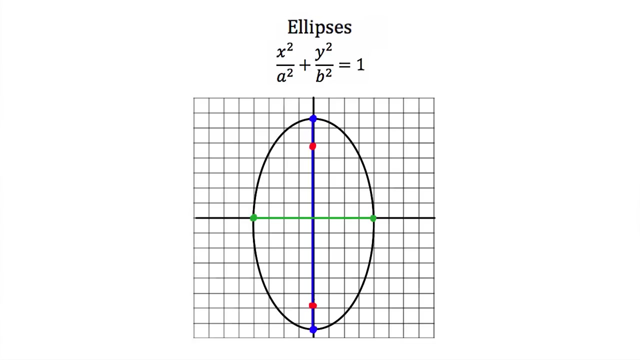 The B term is still underneath the Y so this distance is still B and then this distance is still B. In this example B is greater than A. Therefore our major axis is in the Y direction. In our previous example A is greater than B so our major axis is in the X direction. Now the last thing we have to discuss is how to find our foci. Well from the center to our foci I'm going to call this distance C. Now if our foci are on the X axis or the major axis is in the X direction, then C squared is equal to A squared minus B squared. Notice that our foci are in the X direction from our center and that the A squared term comes first. If our foci are in the Y direction from our center, then this distance is still called C, but defined C we use the equation C squared is equal to B squared minus A squared. 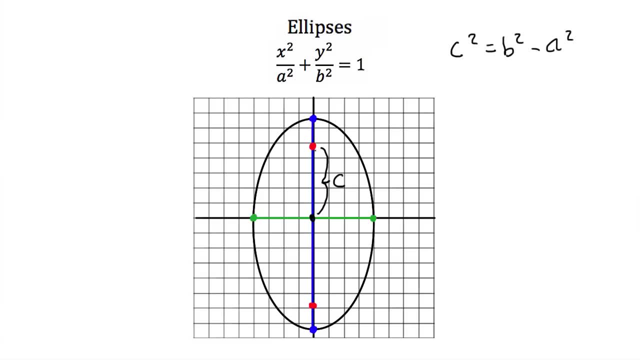 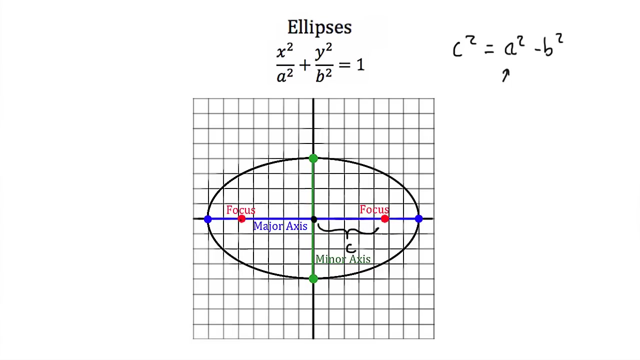 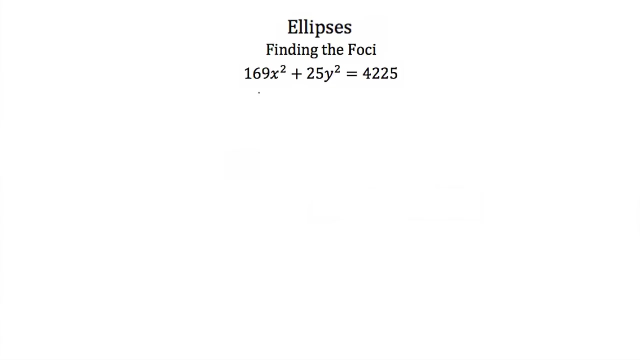 Notice because our C is in the B direction or in the Y direction the B squared comes first in this equation. The way to remember this is that our foci are always on our major axes. If our major axis comes from B being larger than A, then B comes first in our equation. If our foci are on our major axis and that axis is in the X direction, then A comes first in our equation. So let's try finding the foci of this ellipse. This ellipse has the equation 169 times X squared plus 25. times y squared is equal to 4,225. Now this is not in standard form. So to put it in standard form let's divide everything by 4,225. Then we'll end up with x squared over 25 plus y squared over 169 and that's equal to 1. Now this is in standard form. 25 is 5 squared and 169 is 13 squared. So think of this as x squared over 5 squared plus y squared over 13 squared equal to 1 and that means our a is 5 and our b is 13. Now whenever you're dealing withconic sections it's easier to sketch a graph to figure out what you're doing. Step 7. Step 8. Step 7. Step 9. 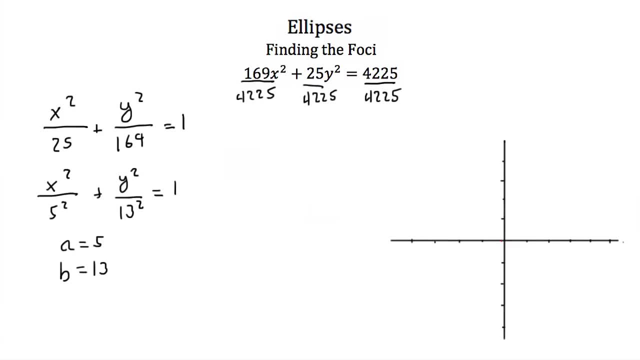 If the center of this ellipse is at the origin, and my A term is 5, that means I have co-vertices, because A is less than B, 5 units from the center in the X direction. 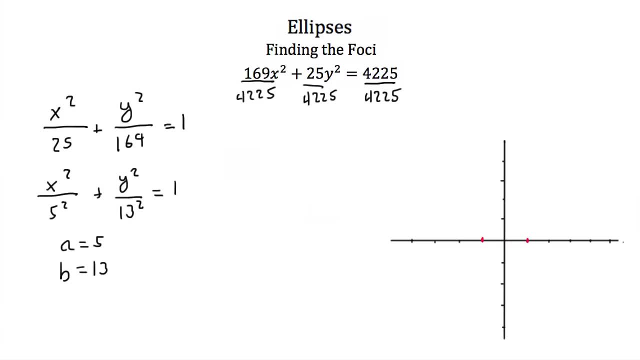 So say it's here and here. My B value is 13, so from that center and in the Y direction, I have vertices 13 units away from the center. So say that's here and there. 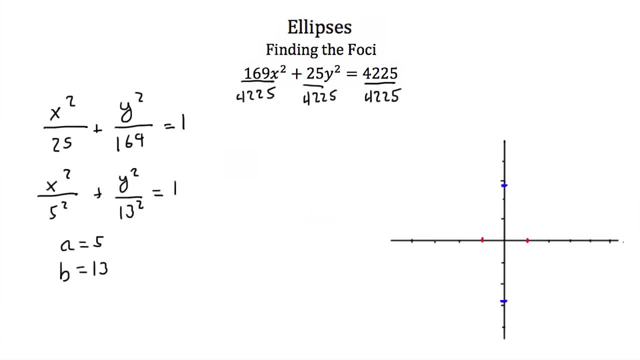 My major axis is in the Y direction, because that's longer than the axis in the X direction, which means my foci are going to be on the Y axis here. My ellipse will look something like this. Now my foci are some C distance away from the center. And because my major axis is my Y axis, then C squared is equal to C squared. So I can easily solve for C. I just plug in 5 for A and 13 for B. I'll have C squared is equal to 13 squared minus A squared, or 5 squared. 13 squared is 169. 5 squared is 25. 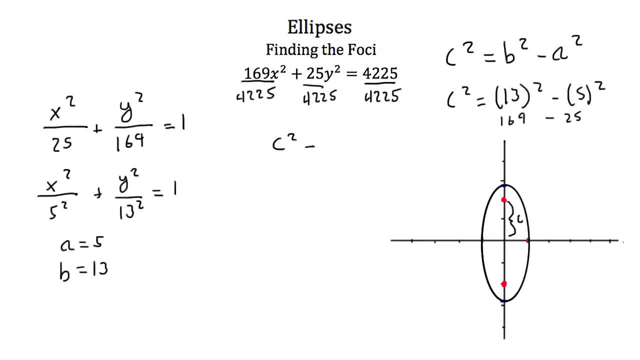 So we're going to get C squared is equal to 144. Take the square root of both sides, and we're going to find out the square root of both sides. And we're going to find out the square root of both sides. So we're going to find out the square root of both sides. So we're going to find out the square root of both sides. And we're going to find out that C is equal to plus or minus 12. But C is a distance. 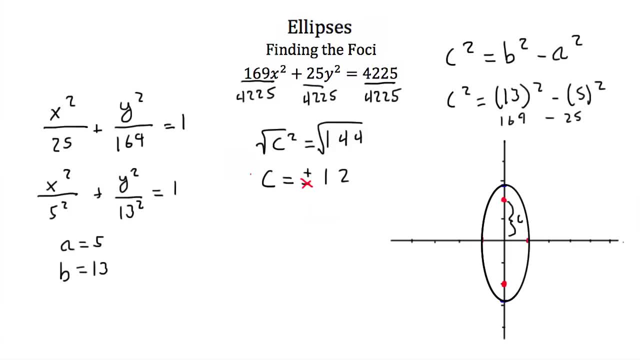 And we can't have a negative distance. So all we have to worry about is that C is equal to 12. 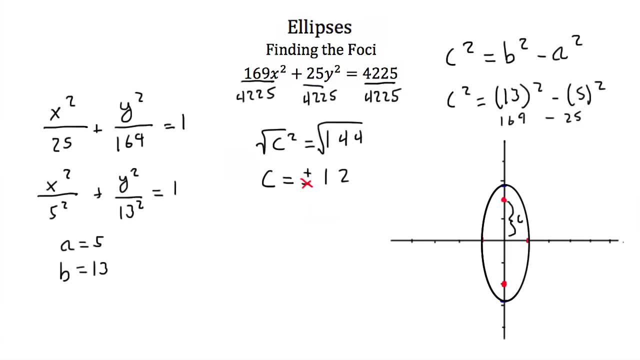 That means that our foci are a distance of 12 along our major axis from our center. Our center is at 0, 0. 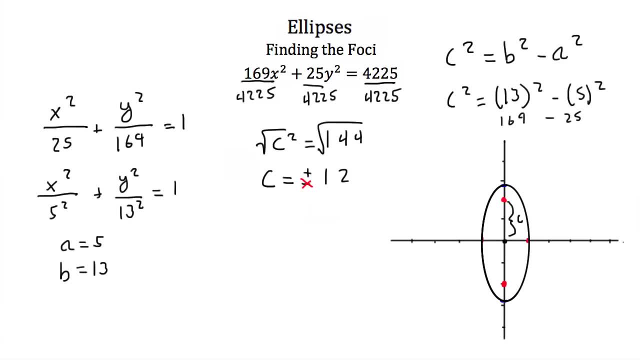 So that means our foci are 12 units above 0, 0, and 12 units above 0, 0. 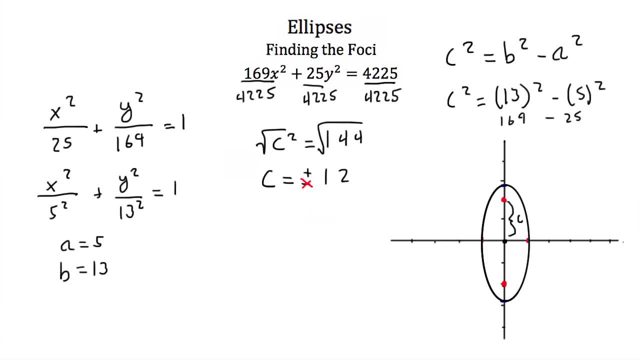 And that means our foci are 12 units above 0, 0, and 12 units above 0, 0. units below 0, 0. So our foci are the points 0, 12 and 0, negative 12. Now let's try 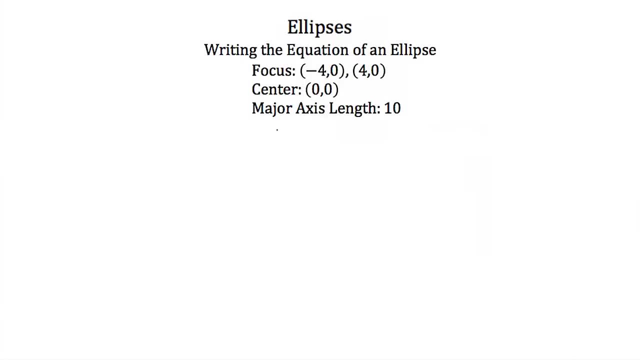 going the other way. Let's try writing an equation of an ellipse given all this information about our ellipse. Its center is at 0, 0 which means we can use the standard form x squared over a squared plus y squared over b squared is equal 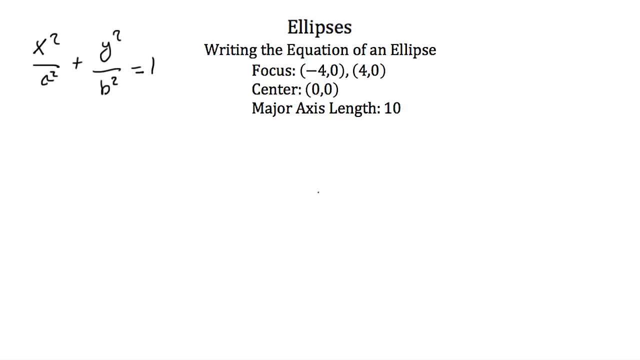 to 1. We're given the location of our foci and we have a major axis length of 10. Now again whenever you're dealing with conic sections it's always easier to sketch a graph. We know our foci are at negative 4, 0 and 4, 0. Let's say that's here and there. 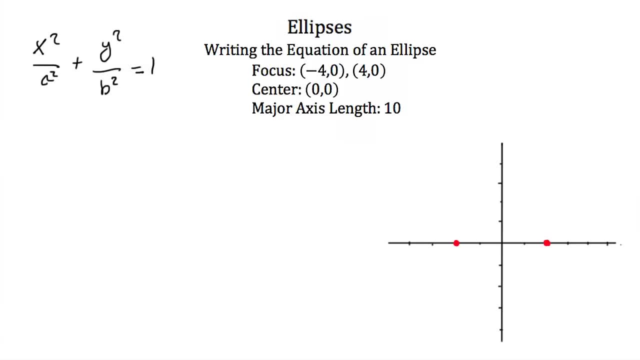 Since our foci are on our x-axis that means our x-axis is our major axis and we're told that our major axis length is 10. So if I have a major axis vertice here and here the distance between these is 10. That means that the distance from this vertice to our center is 5. It also means that that distance is a. So using this information we found our a value a is equal to 5. We also know that if our foci are at 4, 0 and negative 4, 0 then this distance is 4 and this is also my c distance so my c is equal to 4. Now if I'm going to write this in standard form I need my a and my b. But I don't have my a and my b I have my a and my c so I need to find b. I can find my b value by using the equation c squared is equal to a squared minus b squared. I'm using this equation with a squared listed first because my major axis is in the x direction. So if I plug these values into this equation I'll have 4 squared is equal to 5 squared minus b squared. 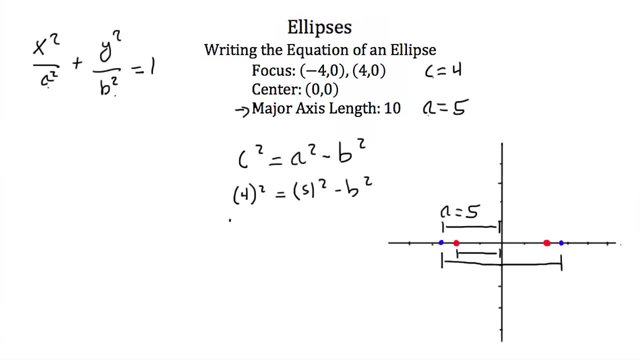 This is 16 is equal to 25 minus b squared. Subtract 25 from both sides I'll have negative 9 is equal to negative b squared or b squared is equal to 9. Take the square root of both sides and ignore the negative answer and we'll get that b is equal to three. 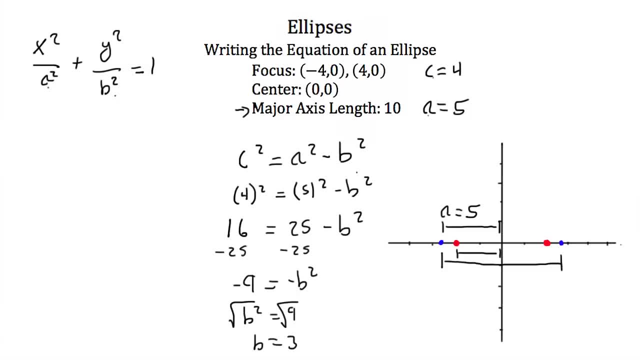 So my equation then if I plug in a and b would be x squared over 5 squared plus y squared over 3 squared and that's equal to 1. Simplify and we have x squared over 25 plus y squared over 9 is equal to 1. That is the equation of our ellipse in 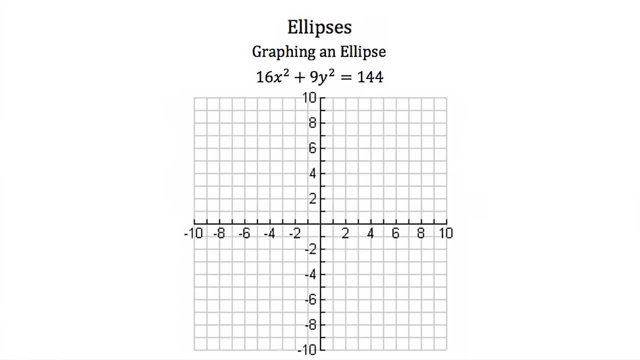 standard form. Now the last thing we have to do is learn how to graph an ellipse. Our equation that we're going to graph is 16 x squared plus 9y squared is equal to 144. Now this is not in the standard form of an ellipse equation. So we're going to put it in the standard form. We're going to take 16 x squared plus 9y squared and that's equal to 144 and we're going to divide everything together. So what we're going to do here we're going to take our ellipse and we're going to 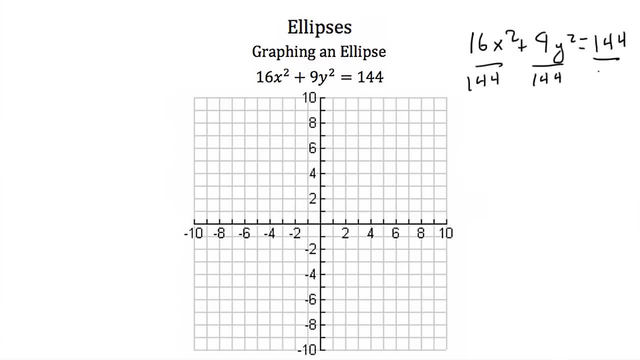 by 144. If I do that I'll have x squared over 9 plus y squared over 16 that's equal to 1. You can also think of this as x squared over 3 squared plus y squared over 4 squared and that's equal to 1. This means that my a is equal to 3 and my b is equal to 4. Now the center of my ellipse is at the origin. My a values are my x values from the center to my vertices in that direction so if we go from 0, 0 and we go to the right 3 we'll have that point there and if we go to the left 3 we'll have that point right there. Our b values are our distance from the center to our vertices in the y direction . 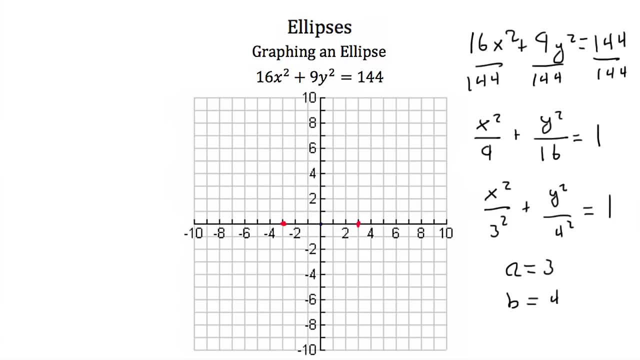 So if we go from 0, 0, up 4, and then down 4, we'll have those two points. And if we connect all these with a smooth curve, our ellipse would look something like that. So that's how you can graph an ellipse. 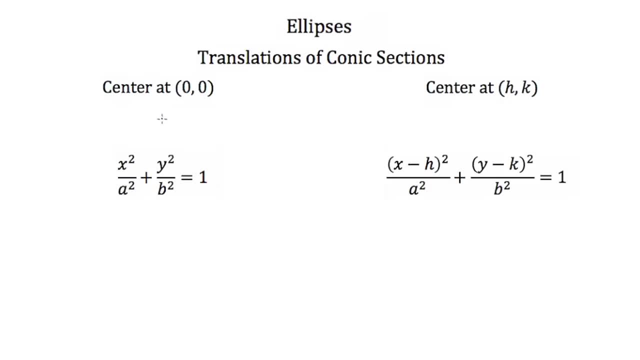 Now so far, all the ellipses that we've been talking about have had their center at 0, 0. And we've been using this equation, x squared over a squared plus y squared over b squared is equal to 1. But what if our ellipse doesn't have its center at the origin? It's got it at some other point. And I'm going to call that point hk. So if I had an ellipse with a center at 1, 2, that would mean h would be 1 and k would be 2. 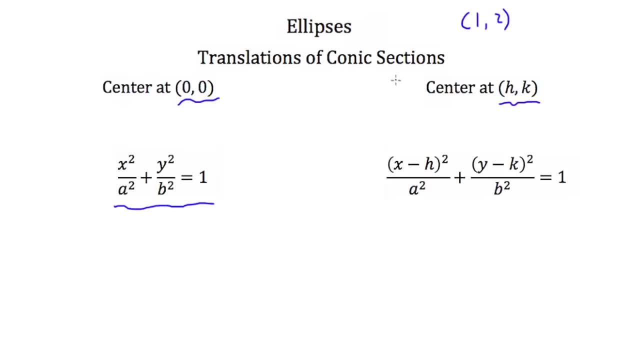 Well, if our ellipse has some other point at the origin, some other center than the origin, then we use this equation right here. 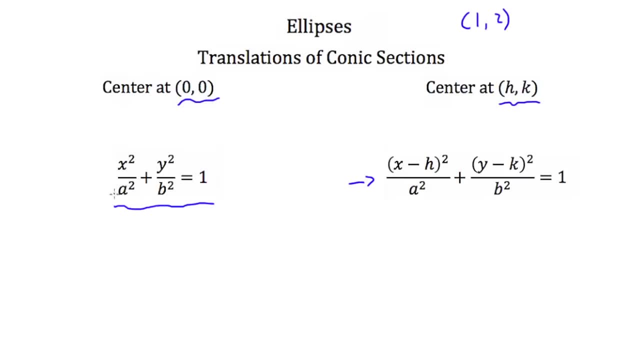 And the easiest way to memorize this equation is that everywhere you had an x before, we now have an x minus h. Everywhere you had a y before, you now have a y minus k. And h is the x coordinate of our center, and k is the y coordinate of our center. But our a and our b values are exactly the same. 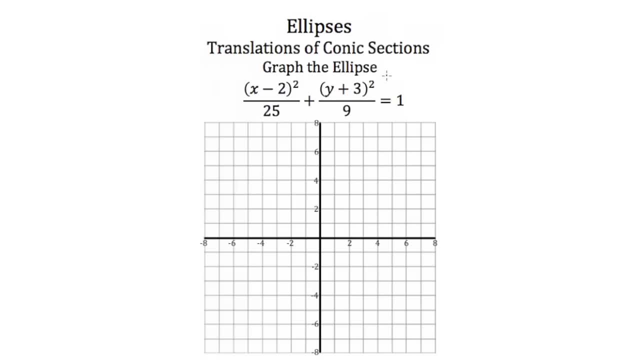 So let's try graphing this ellipse. Here we have an equation in standard form, x minus 2 squared over 25 plus y plus 3 squared over 9 is equal to 1. This is the standard form of x minus h squared over a squared plus y minus k all squared over b squared is equal to 1. 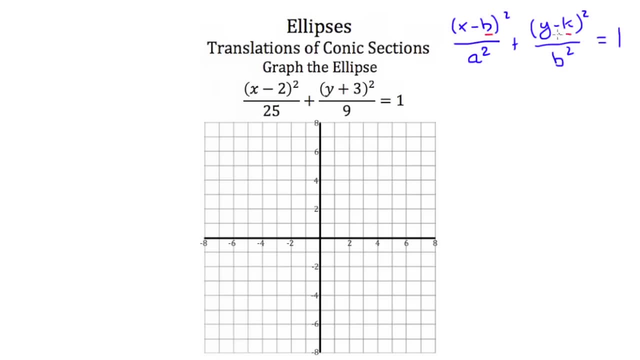 Now remember, h and k are the coordinates of the center of our ellipse. 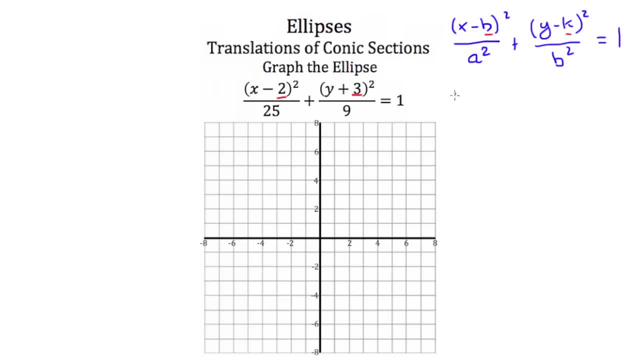 So right away we can find the center of our ellipse. That's at the point 2 and negative 3. 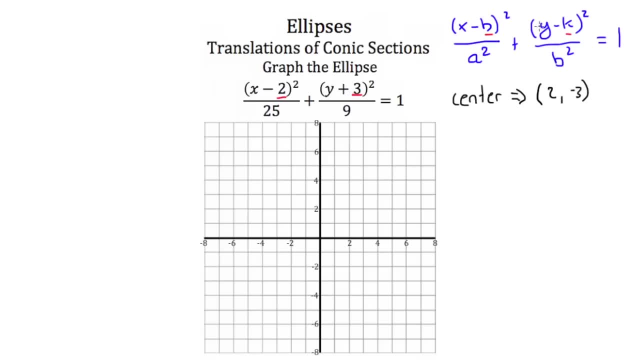 It's negative 3 because this is a minus k in our standard equation, and this is plus 3. 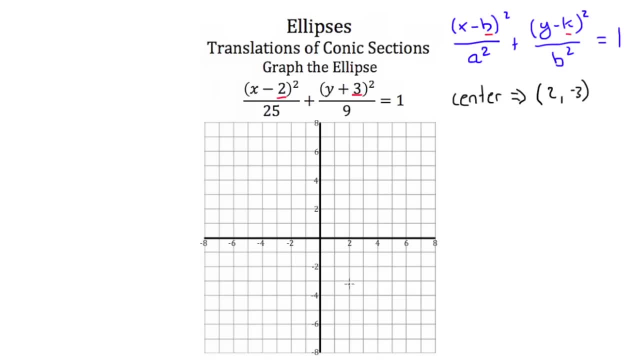 So the standard equation is like this. The center of my ellipse is at 2, negative 3, which is right here. 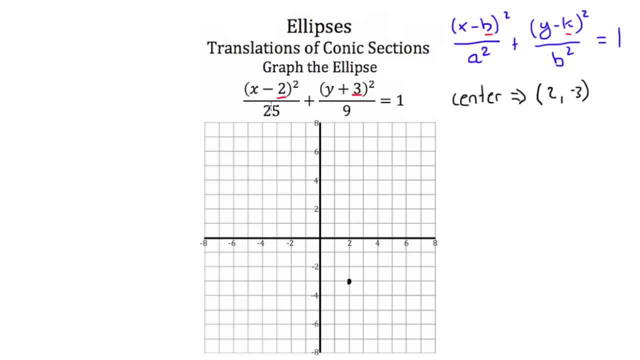 And now I can look at my a and my b values. My a value is the number underneath the x term, so my a value is here. I have a squared is equal to 25, and that means a is equal to 5. 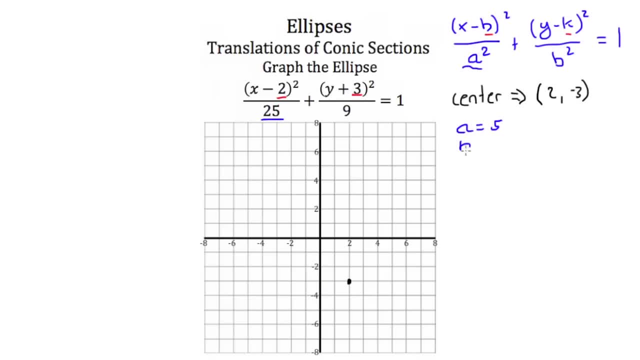 b squared then is equal to 9, and that means b would be equal to 3. Now our a squared term is underneath our x term, which means we have vertices for this ellipse in the x direction and a value away from our center. 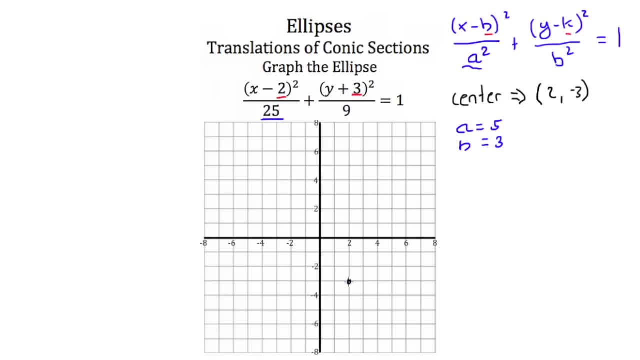 So a is 5, so if I go to my center at 2, negative 3, and I go to the right 5 units, I will run into one of the vertices of my ellipse. And if I go in the negative x direction, I'll run into another one. 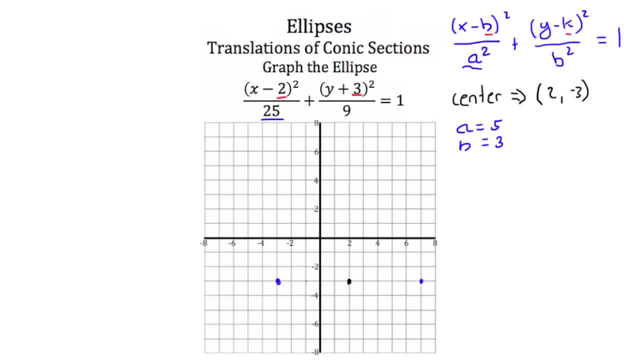 I can also find my minor axis vertices. My b value is 3, and my b squared is underneath my y term. So that's my change in y, or the distance I'll find my vertices, or my co-vertices. So I go to my center and I go up 3, because b is 3, and then I go down 3 from the center, and I'll find my minor axis vertices. The last thing I have to do are find my foci. 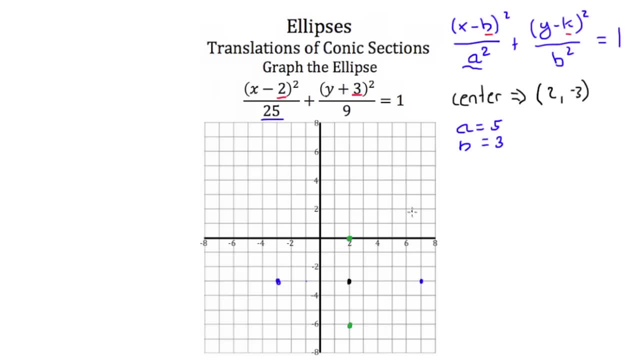 My a squared term is larger than my b squared term. So I use the formula c squared is equal to a squared minus b squared. 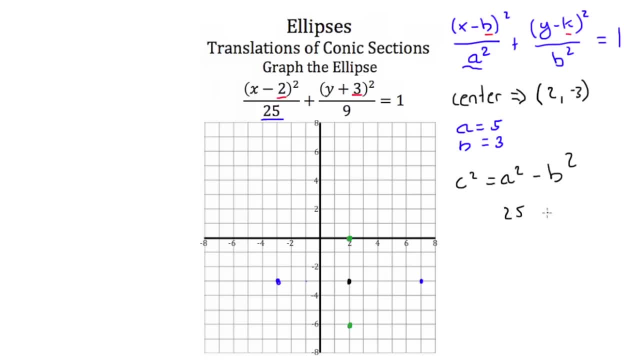 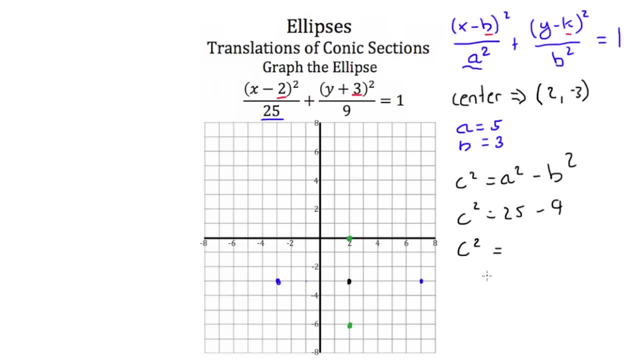 is equal to 25 minus 9 or you can say C squared is equal to 16 and that means C is equal to 4. That means our foci are a distance of 4 away from our center and 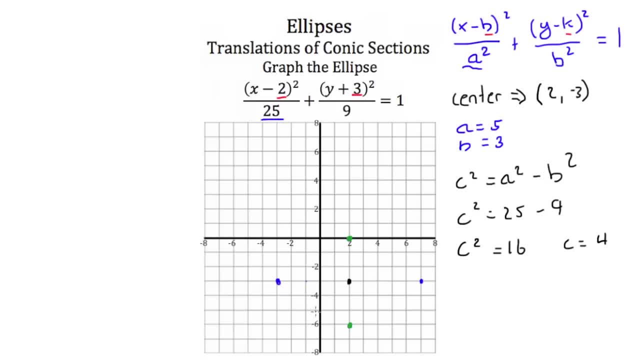 they're along our major axis which is this axis here that moves in the X 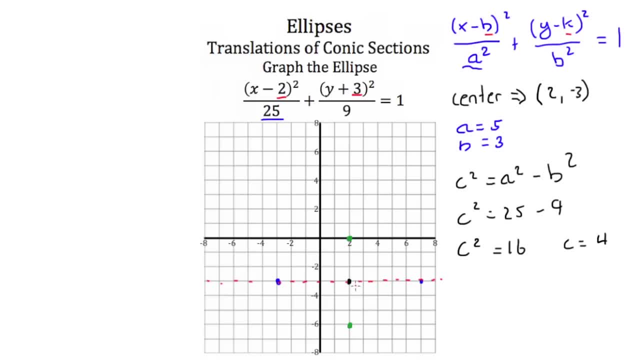 direction. So I go to my center and I count off 4. I find a focus right there and then another one right here and that means our ellipse should look something 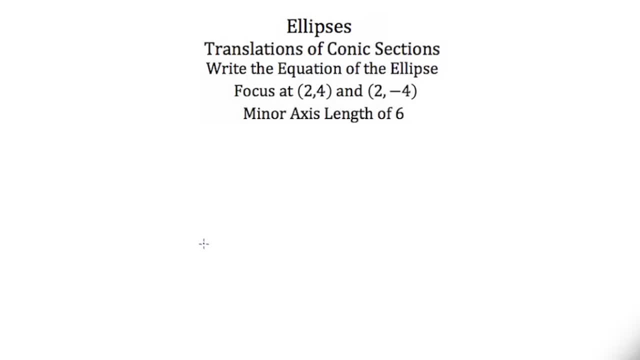 like this. So let's try another problem. Here we're told to write the equation of the ellipse and then we're told it has a focus at 2 4 and 2 negative 4 and a minor axis length of 6. 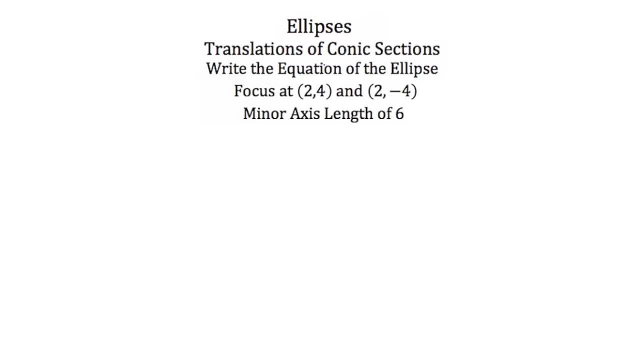 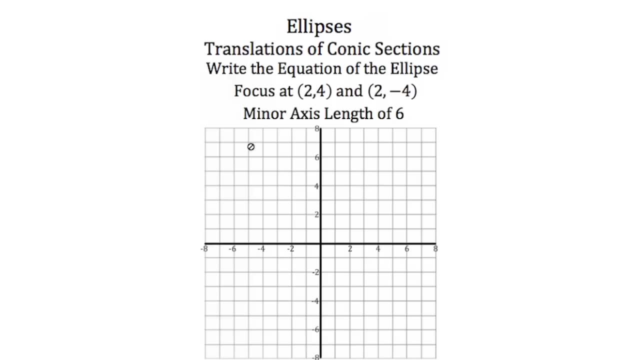 Well whenever I'm doing conic sections I always like to draw a picture. So let's plot the points that we're given. We have a focus at 2 4 and 2 negative 4. Now these are our foci and that means our major axis would be in this direction. And our major axis would be here and that means our major axis would be in this direction. Now these our foci and that means our major axis would be in this direction. Halfway between our two foci, we would find the center of our ellipse. Halfway between 4 and negative 4 would be 0 in the y, so the center of our ellipse is right there. Our center, that's the point 2, 0. 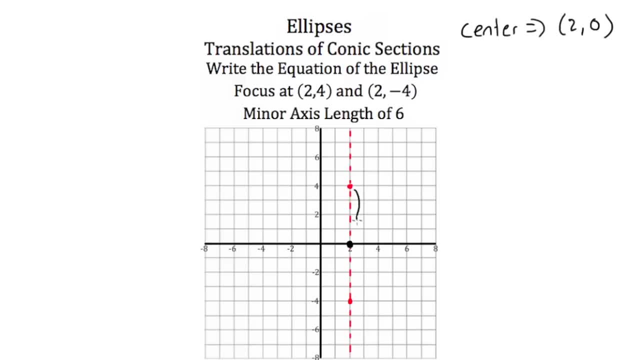 And that means that this distance here is 4, and that tells us that our c value is 4. 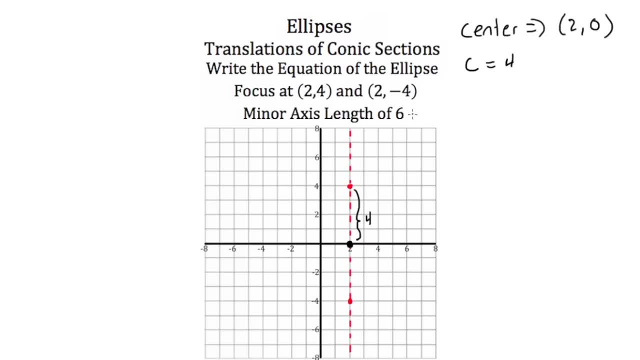 Then we're told that we have a minor axis length of 6. 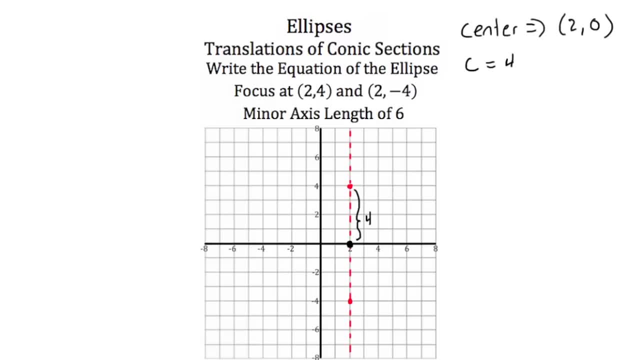 Well, if the entire axis length is 6, then half of that axis length would lead us from the center to one of our minor axis vertices. So our minor axis vertices... Our co-vertice would be 3 units away from our center. So if I go to the center, and I go perpendicular to our major axis, 3 units, I'll find a co-vertice, and then in the other direction, another one. And this distance is 3. Now this distance is in the x direction, and that tells us that our a value is 3. Well, my equation of my ellipse, which does not have its center at the origin, has its center at some other point, in this case 2, 0. 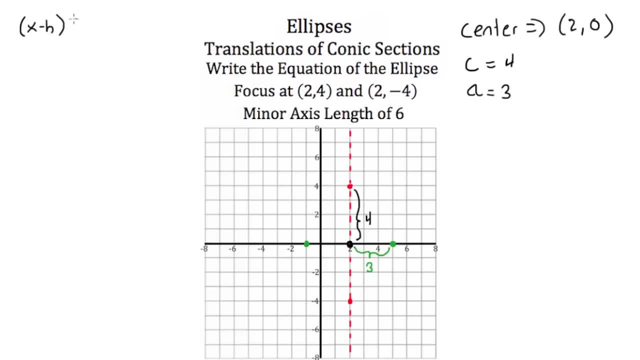 That equation looks like x minus h squared over a squared plus y minus k squared over b squared is equal to 1. Now I know my h and k, they're just 2, 0. I know my value of a, that's 3. The only thing I'm missing is my value of b. Well, I can find that because I have my c value. Now remember, our major axis is in the y direction. That's our longer axis, which means c squared is going to be equal to b squared minus a squared. If I plug in 4 for c, that's equal to b squared minus 3. 3. 3. 3. 3. 3. 3. 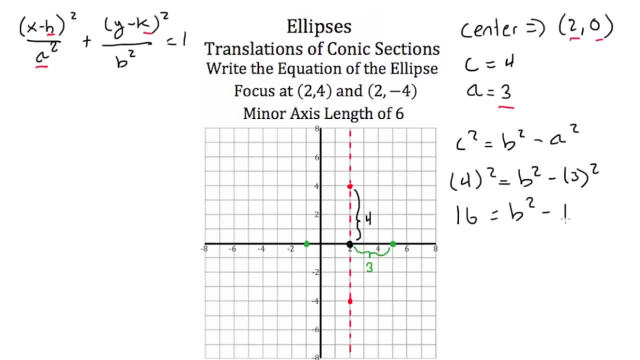 Come up with 16 is equal to b squared minus 9. Add 9 to both sides. 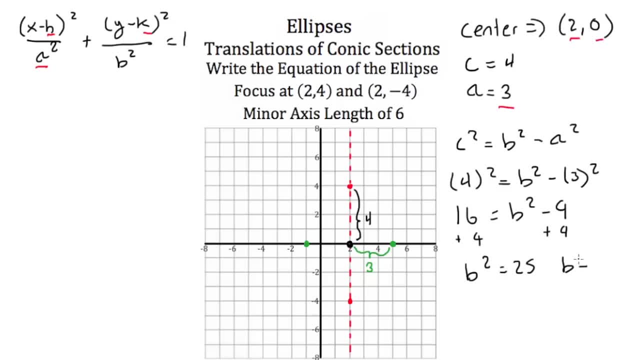 And we'll get b squared is equal to 25, and that means b is equal to 5. 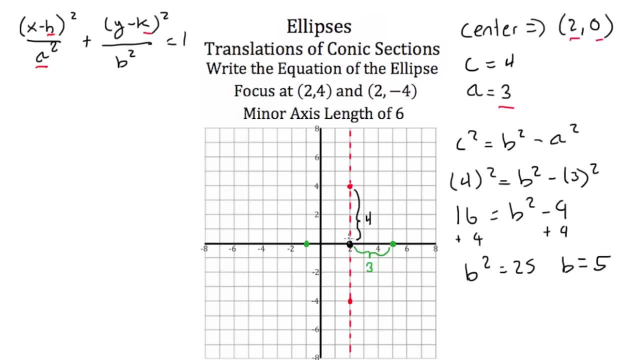 Now if I want to, I can go 5 units along my major axis from my center and find my vertices. But I don't really need it. All I needed was my. 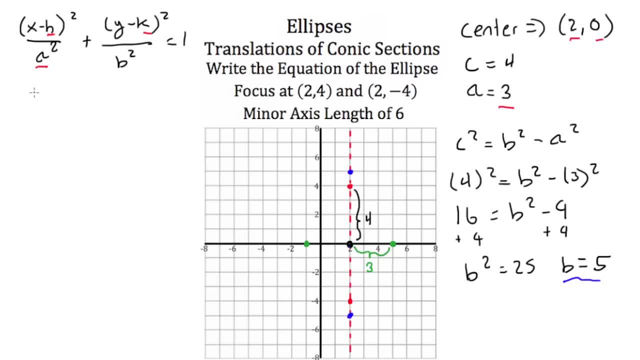 value of B so if I plug all that in to this equation I get X minus H now H is 2 so X minus 2 squared over a squared a is 3 and if I square that I get 9 plus y minus k squared k is 0 so it's not y minus it's just y but it's still squared and that's over B squared now B is 5 so 5 squared is 25 and that's equal 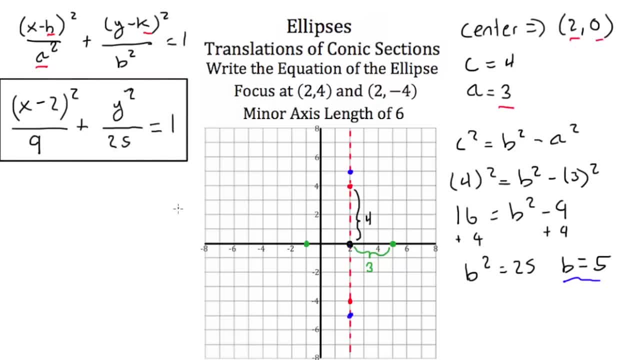 to 1. So this is the equation of an ellipse with its focus at 2 4 and 2 negative 4 and a minor axis 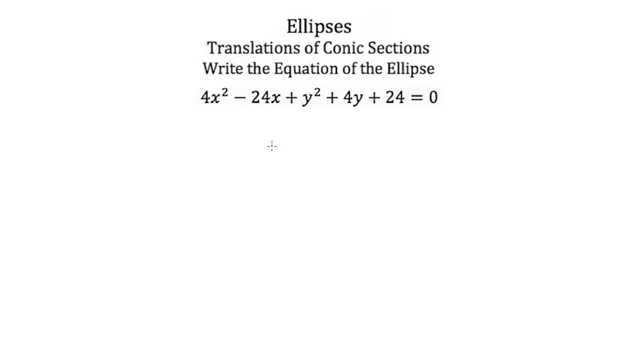 length of 6. Now we have one more problem to try. Here we're asked to write the equation of the ellipse and then we're given this equation here 4x squared minus 24x plus y squared plus 4y plus 24 is equal to 0. Now this is most likely an 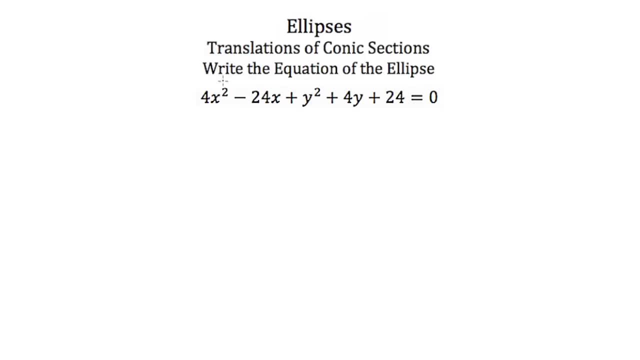 equation of an ellipse because we have an x squared and a y squared. But then we have these linear terms here 24x and 4y so somehow we're going to have to put 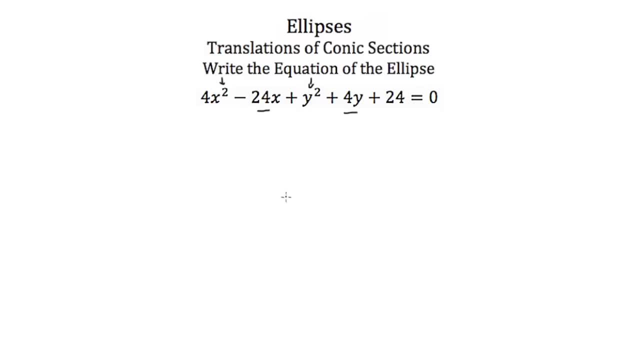 this into the standard form equation. Now the way to do this is to complete the square. We'll start with the x's here. If I have 4x squared minus 24x, first thing 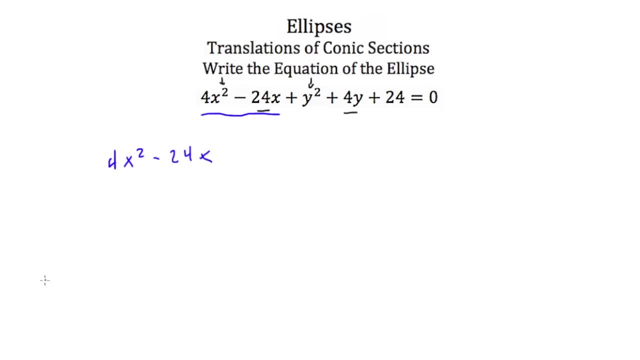 I want to do is factor out a 4 which means 4 times x squared minus 6x would be in the inside. Then looking at the y's I'll have plus y squared plus 4y and I'm going to have to complete the square for the y's as well. The last thing I'm going to do is subtract 24 from both sides so this will all be equal to negative 24. Now looking at this x squared minus 6x I want to complete the square for this so I take half of this 6 which would be negative 3 and I square it. That would give me 9 which means I'm going to want to add 9 inside these parentheses to make what's inside these parentheses a perfect square. 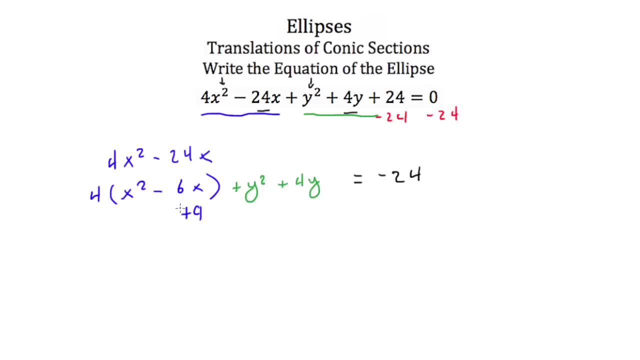 But if I add 9 inside the parentheses I'm actually adding 9 times 4 because everything inside these parentheses is being multiplied by 4 so really I'm adding 36 to the left-hand side of this equation which means I have to add 36 to the right-hand side of this equation. Then I'm going to look at this y squared plus 4y. If I take half of this 4 I'll get 2 and square it I get another 4. So I want to add 4 to this group and this group didn't have a greatest common factor. It's not multiplied by anything like the x's were multiplied by this 4 so I don't have anything to multiply this 4 by. But again since I added 4 to this left-hand side I have to add 4 to the right-hand side. 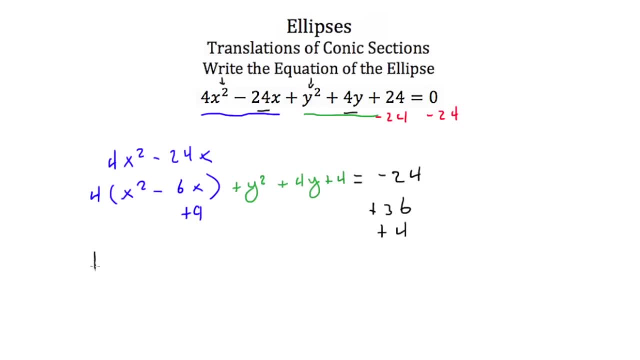 So what I have now is 4 times x squared minus 6x plus 9 plus y squared plus 4y plus 4. That's equal to 16. Now this x squared minus 6x plus 9 remember we completed the square which makes this a perfect square. So I can write this as x minus 3 squared if I factor this. And it's still multiplied by 4. I also completed the square for the y variable which makes this a perfect square and I can write this as y plus 2 squared. These are still added together and they're still equal to 16. Now remember I'm trying to get this into the standard form of an ellipse which looks like x minus h squared over 8. 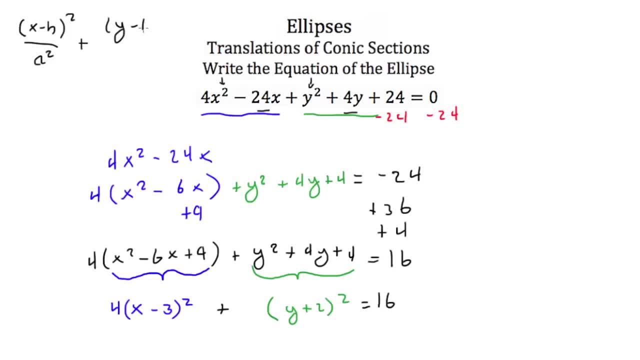 So I'm getting y minus h squared plus y minus k squared over b squared is equal to 1. And I'm almost there. I just have to get this right-hand side equal to 1. So I divide everything by 16. This becomes 1 which is what I want. And I have a 4 in the numerator and a 16 in front of these x's so this will reduce down to just just a 4 in the denominator. So my equation then is x minus 3 squared over 4 plus y plus 2 all squared over 16 is equal to 1. So that's how you use completing the square to rewrite an equation of an ellipse that looks like this into standard form. And that completes our tutorial on ellipses as conic sections.